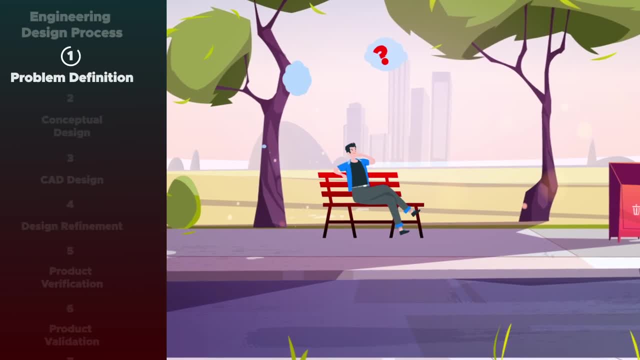 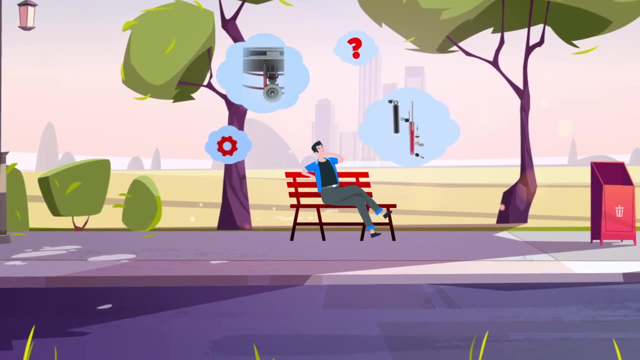 can we improve the ride quality of a truck suspension system? One solution can be found by adding a shock absorber between the chassis and the wheel assembly to absorb or dampen the compression and rebound of the spring. In short, the engineering design process begins by defining a problem and completing 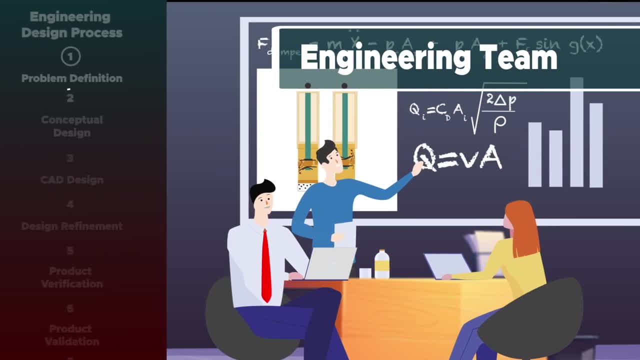 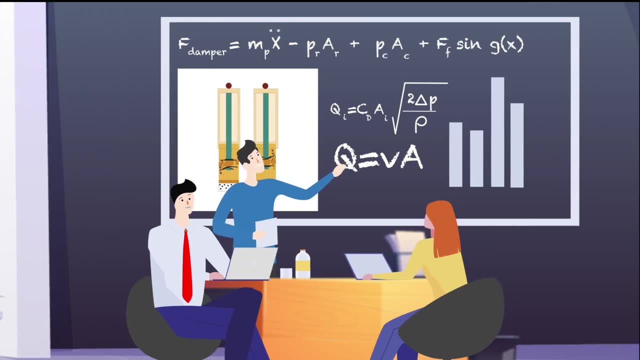 background research on the problem. The second step will be the conceptual design. This is the phase of development where the engineering team and designers work to understand any design issues and find a solution. It is one of the earliest phases of development and usually involves creating a number of solutions so that the direction of the design can be slowly. 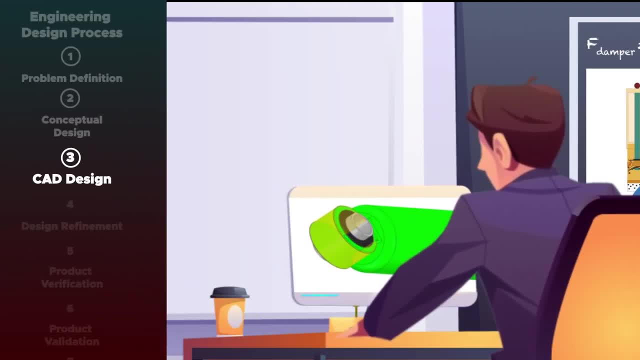 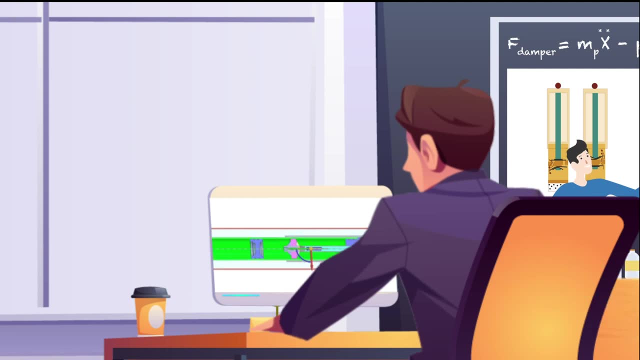 narrowed down. In the third step of the process, the 3D modeling of the product will start using the software. CAD is a type of computer software that is used to create 2D and 3D models and designs. CAD design drawings give valid and accurate details of the design, For instance: 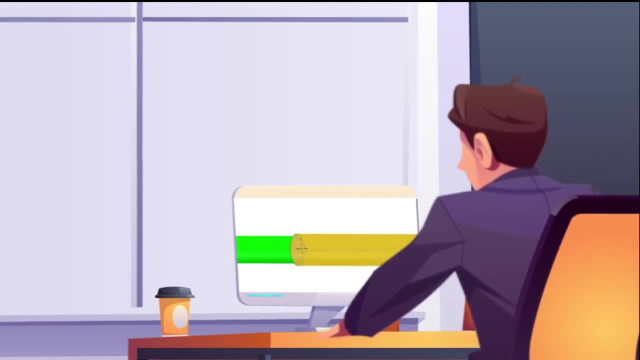 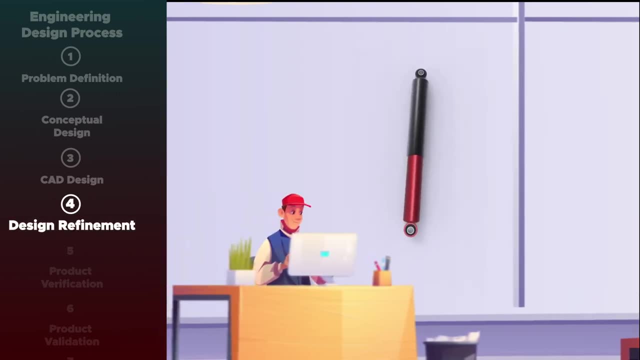 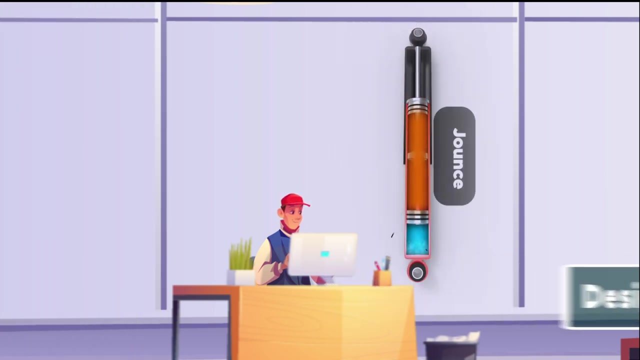 they provide precise dimensions of the shock absorber design, show the inner components of the product and include all necessary drafts with technical details of the design. During the design refinement stage of the design process, all of the individual parts, arrangements, dimensions and surface characteristics are determined by the design engineer. Additionally, 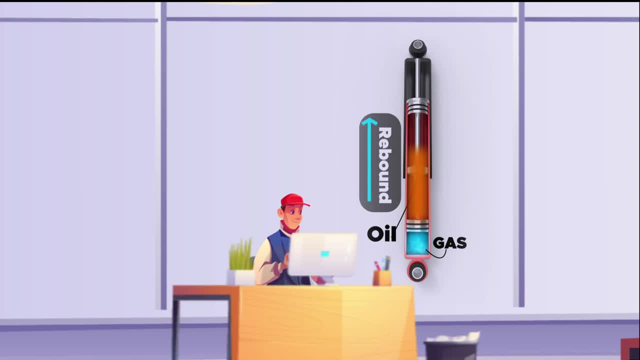 materials are specified, production possibilities are evaluated, costs are estimated and all drawings and other production documents are created, For instance, the orifice size for the rebound valve is determined and the material selection for the shock absorber components is defined. It is important to note that the design is not finalized until all the engineering design. 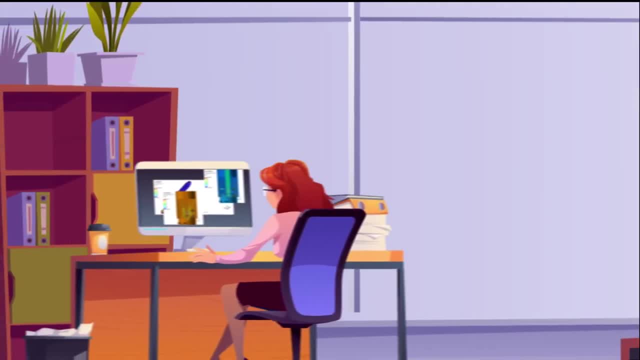 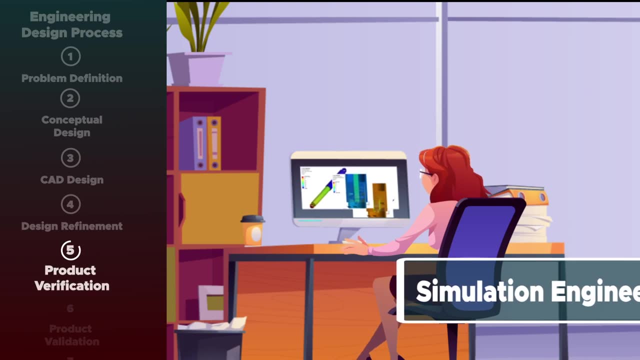 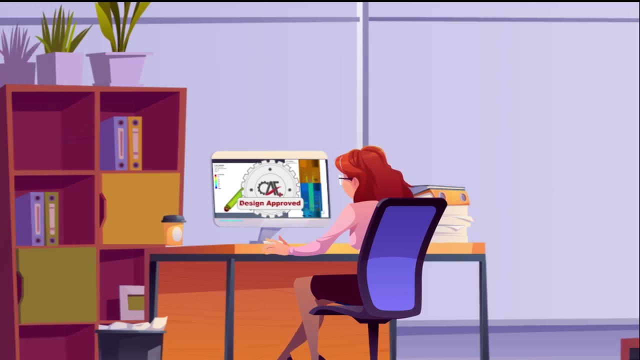 processes are completed. Design verification is an essential step in the development of any product. In this step, the necessary engineering simulation models will be developed and run with high-performance computers to verify the intended function of a product and if it meets the engineering set criteria. Different types of computer-aided engineering simulation: 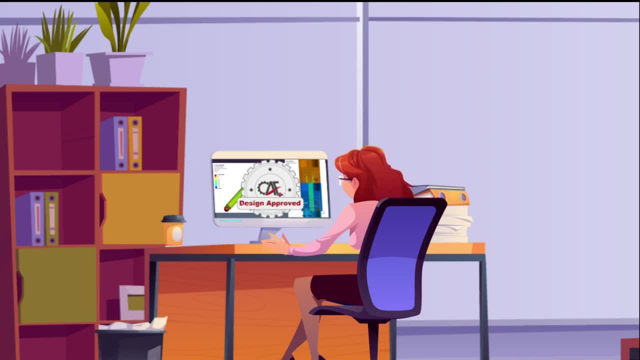 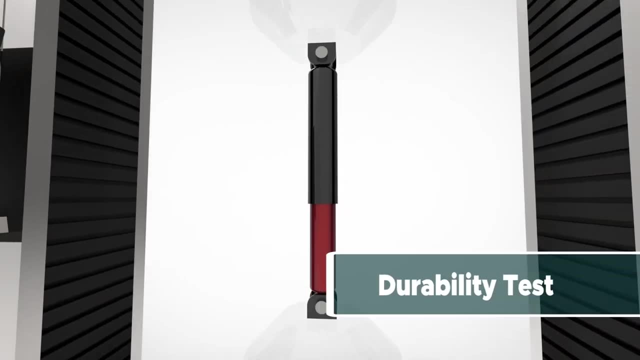 modeling will be conducted depending on the design, such as finite element analysis. Also, a significant number of design problems can be detected in this step. Before going into mass production, it is necessary to build a prototype of the design that mimics the finished product. 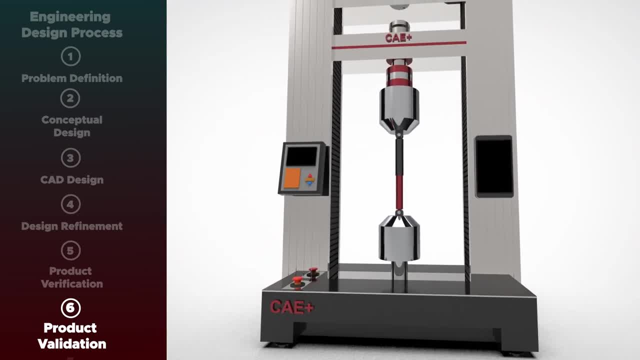 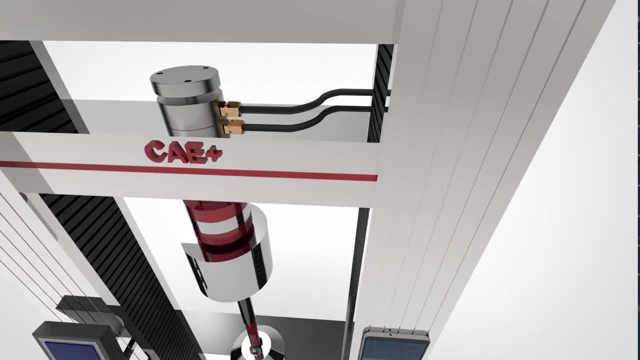 Next, the prototype will go under the design validation phase to validate the product's intended function and requirement performance. For our example, the shock absorber must undergo an accelerated life testing or fatigue test to ensure its durability throughout the intended lifespan of the product. Meanwhile, special tests: